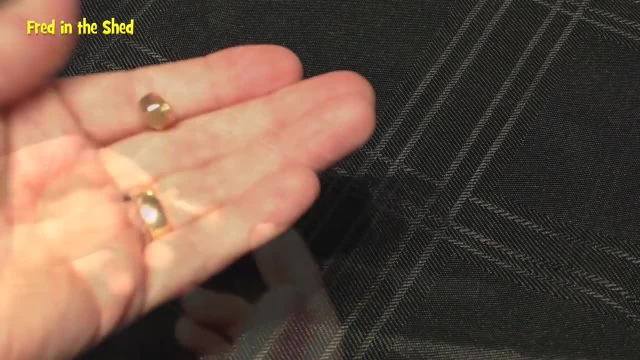 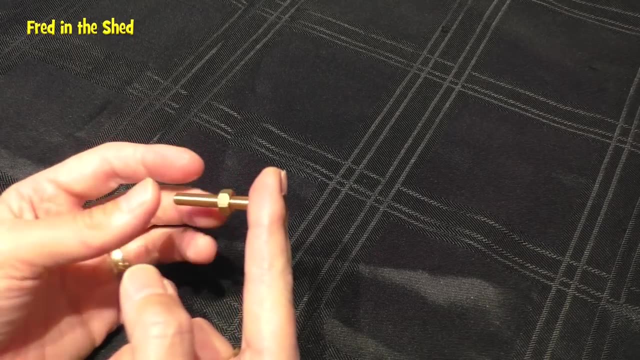 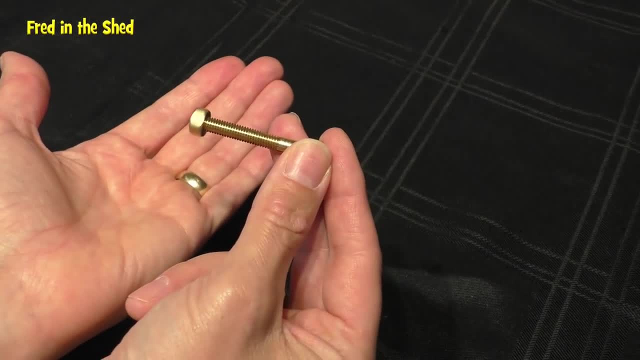 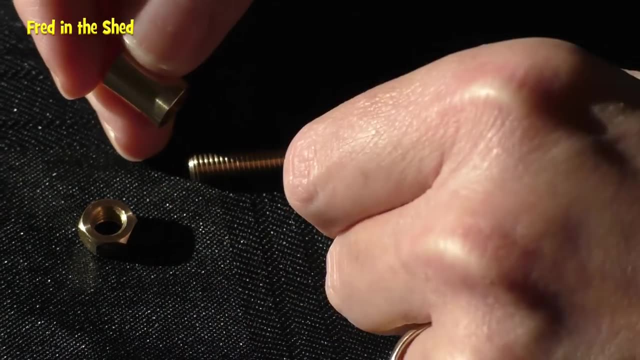 nut will just unscrew itself and fall off, And this is such a cool trick, But it's now time to stop that background music and let me show and explain how the trick works, Right, okay, as you're watching this, you'll notice there's a component I didn't show you at the 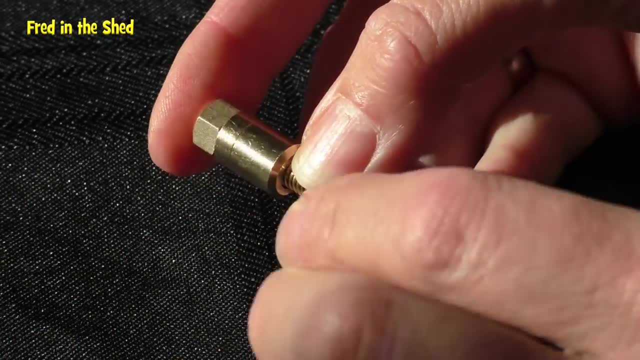 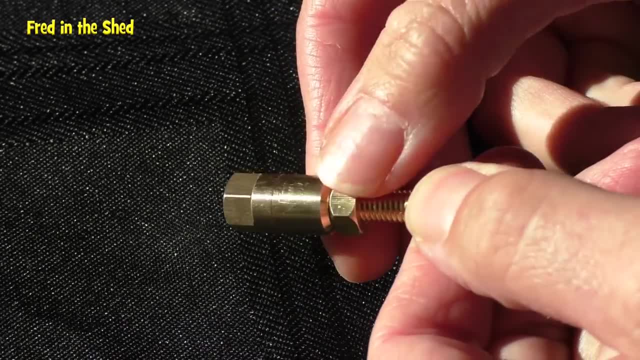 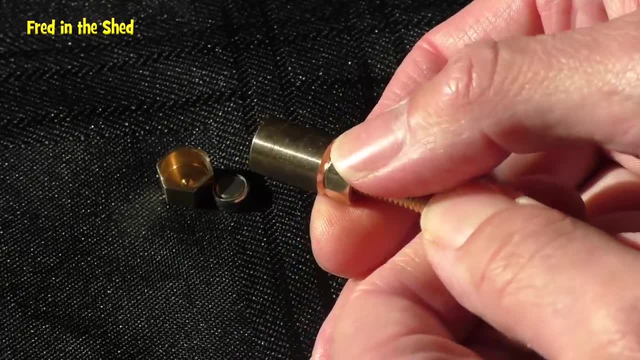 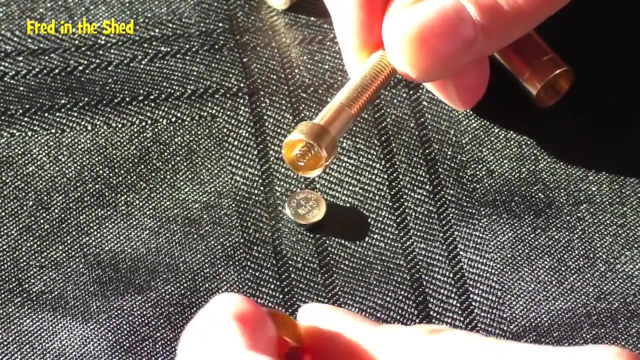 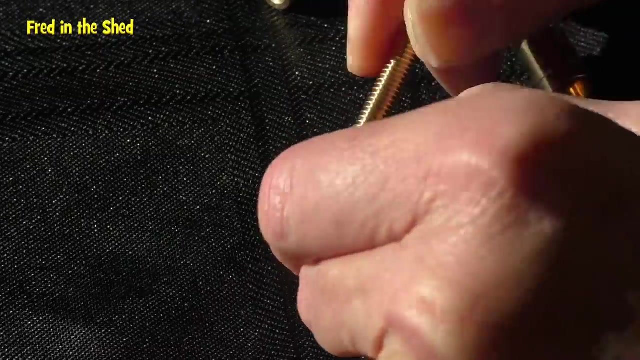 And as you tighten this, just watch what happens to the head of the bolt. It pops off. and here reveals the trick, because inside the head of the bolt itself is a very tiny little watch battery cell And this powers a small magnetic little rotating motor that's built into the 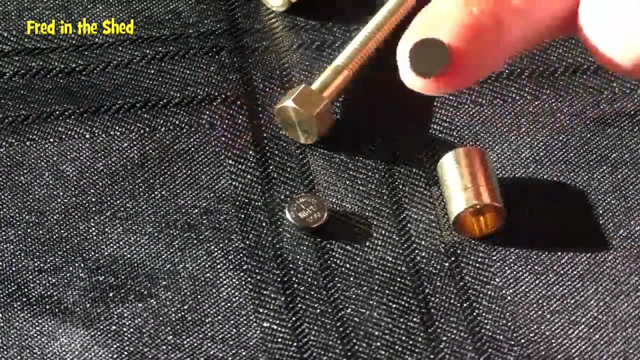 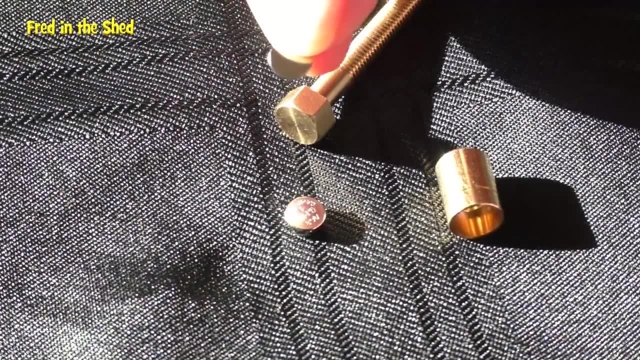 shaft of the bolt And you also get a very, very small neoprene magnet with a little bit of adhesive on it and that sticks to your finger, And when you offer that up to the bolt, the motor starts to turn, it vibrates and the nut comes off. 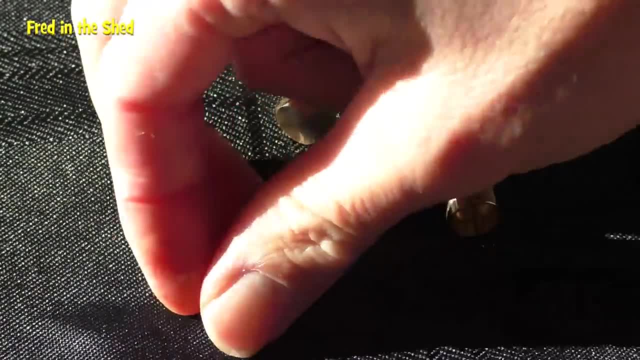 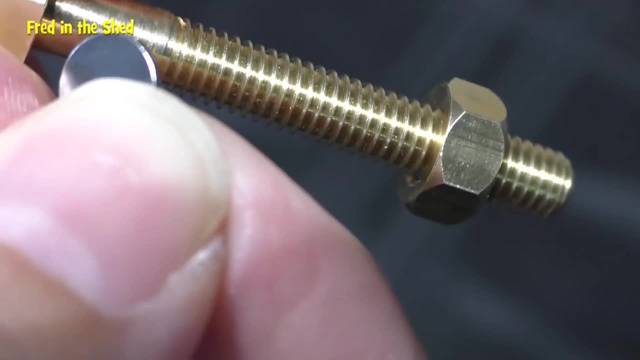 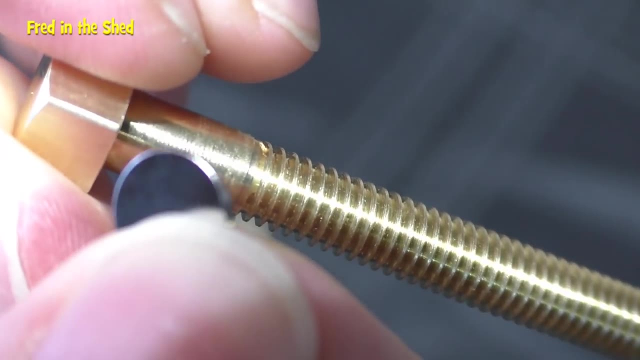 Now, do you remember? at the beginning I said this was an easy trick with one condition. Well, here is that condition. You see, the bolt makes a small vibrating noise. Have a listen And you know. that's the only difference, The downside to this trick. it's not a trick that you can perform in a very sort of quiet. 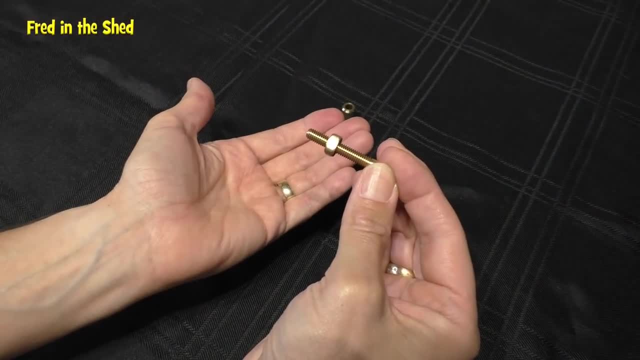 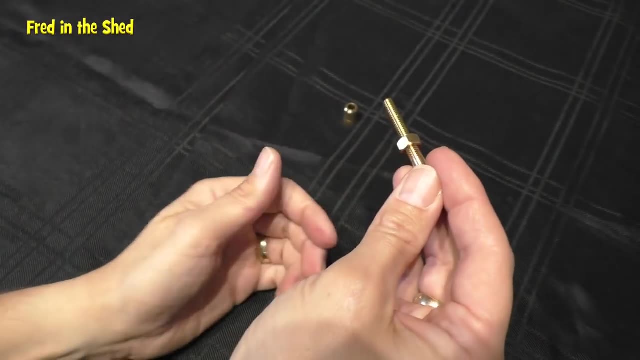 room. It's probably best to do it, say, at a party or something where you've got background noise, people talking, And if possible, you know, sort of take a step back away from your audience, which will help disguise the noise sort of even more. It's not particularly loud. 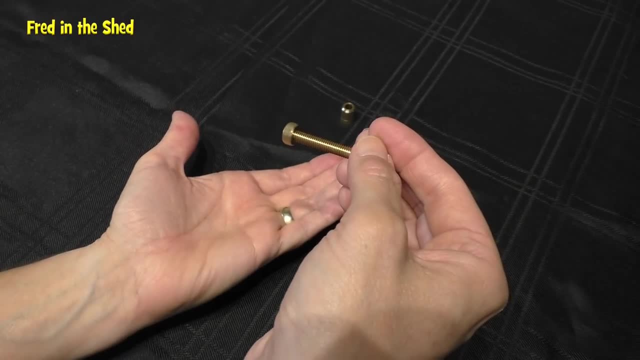 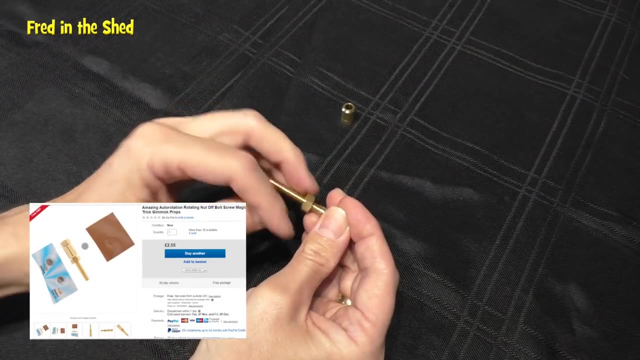 but it would be heard in a quiet environment. So there you go, Something a little bit different on threading a shed one. I hope you enjoyed it. If you did, please give the old video the thumbs up. That helps me and that helps.